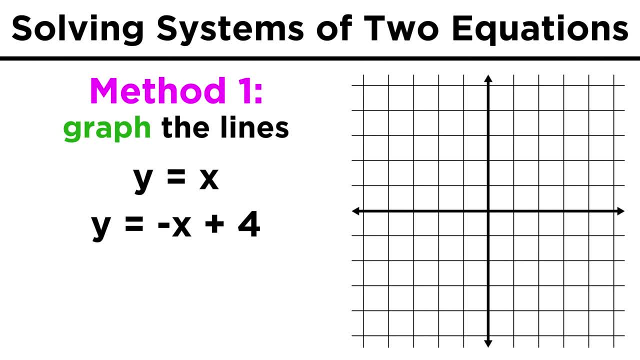 Say we have Y equals X and Y equals negative X plus four. If we place both of these lines on the coordinate plane, we can see that they do indeed cross. If one line represents all of the pairs and X and Y values, then we can see that they. 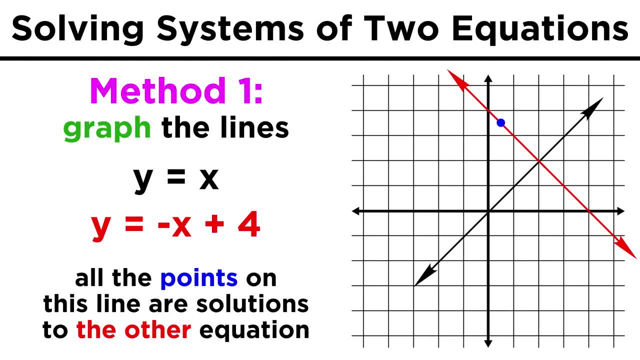 are solutions to one equation and the other line represents all the pairs of X and Y values that are solutions to the other equation, then it must necessarily be the case that the point where they cross must be a solution to both equations, because this point is on. 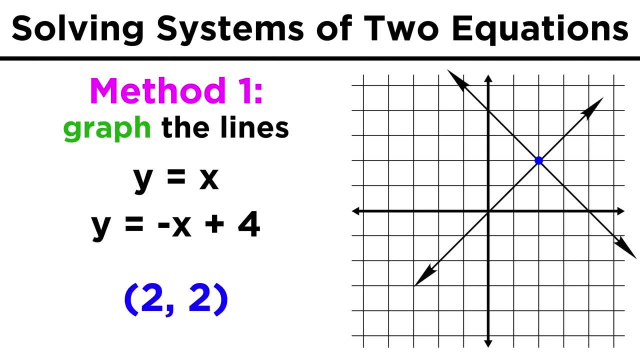 both lines. We can find this solution graphically if our graphs are very neat and tidy or if we are using a graphing calculator, Because, as long as the graph is accurate, we can just observe that the lines cross at the point and therefore X equals two and Y equals two represents the solution. 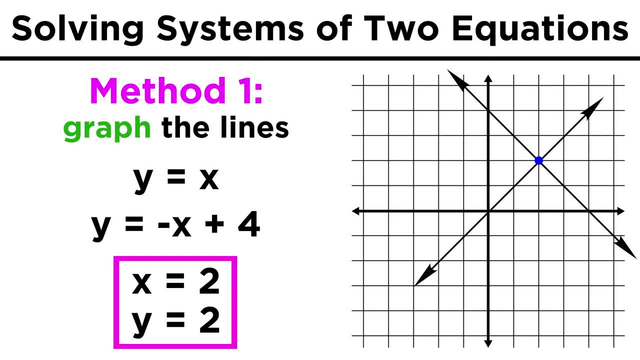 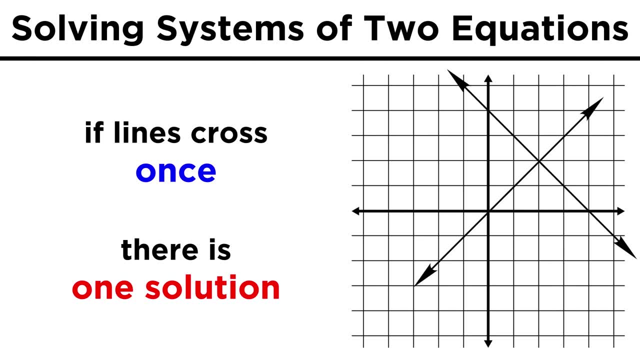 to this system of linear equations. Most of the time, two lines will cross precisely once, and there will therefore be one unique solution to the system. However, other situations include parallel lines Which never cross, so there will be no solution to the system. 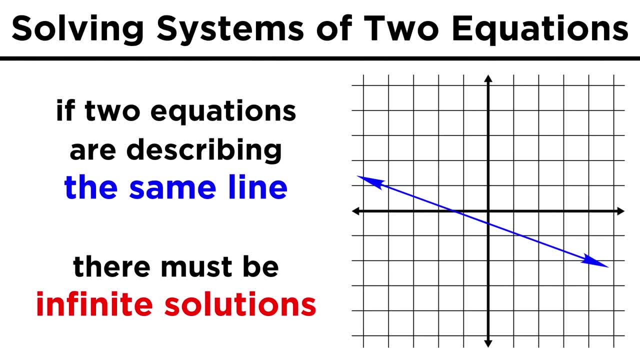 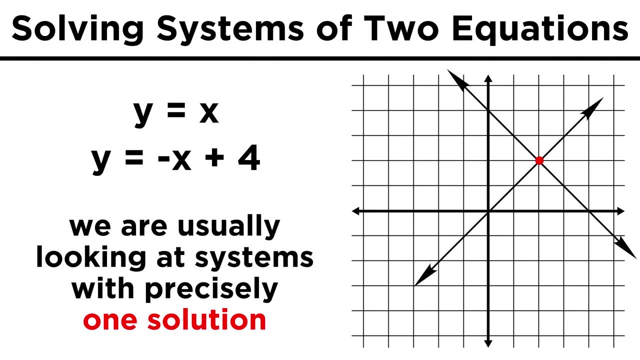 And we could also have two different equations that describe precisely the same line, in which case there are infinitely many solutions, as every point on the line will be a solution for both equations. But, as we said, we are typically concerned with situations where two lines cross once. 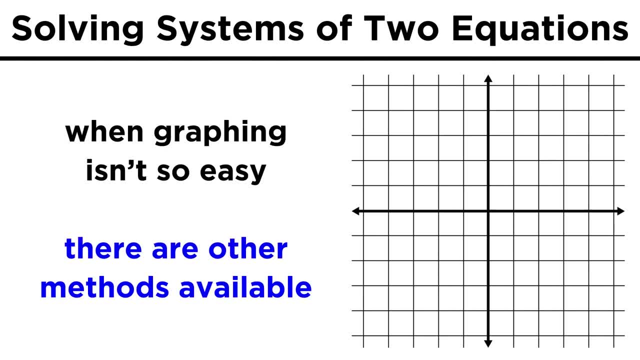 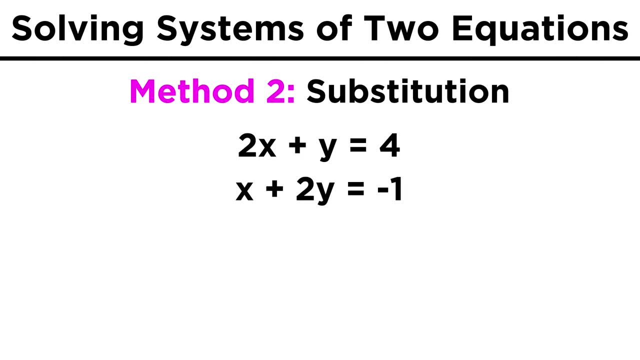 and we want to be able to get that one solution. When graphing isn't so easy for one reason or another, there are other methods we can use to find the solution. The first technique we will look at is called substitution. Say we have these two equations: two X plus Y equals four, and X plus two Y equals negative. 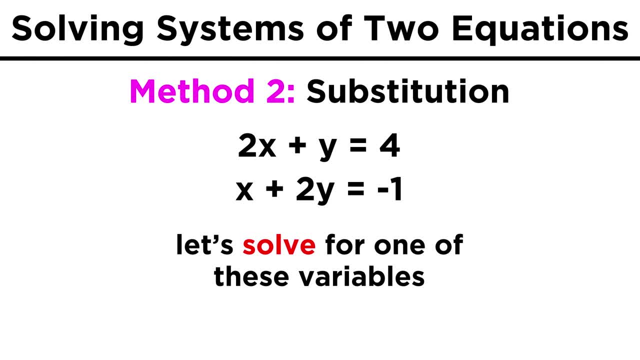 one. What we could do is solve for one of these variables in terms of the other. For example, let's solve for Y in the first equation, Subtracting two X from both lines. we can solve for Y in terms of the other. 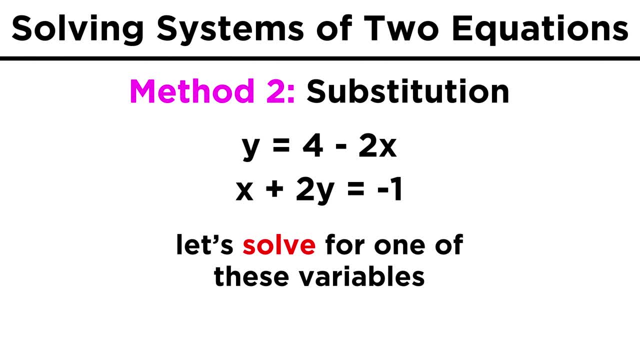 Subtracting two X from both sides gives us Y equals four minus two X. Now what we can do is substitute this value of Y for the Y in the other equation. That means instead of Y we insert the quantity four minus two X. Now we have a new equation with only X, which will make it possible to solve for X. 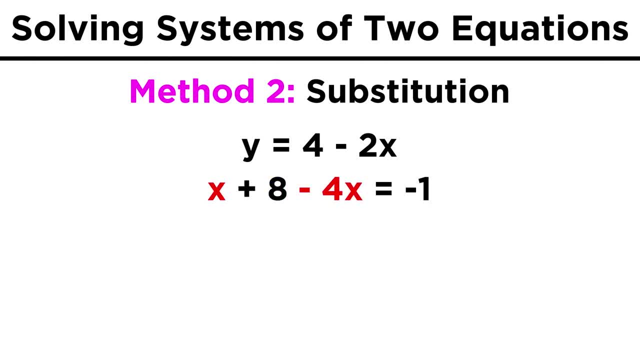 We distribute the two to get eight minus four. X combine like terms, bring the eight to the other side And we get negative three. X equals negative nine or X equals three. That means three is the X coordinate for the point where these lines cross. 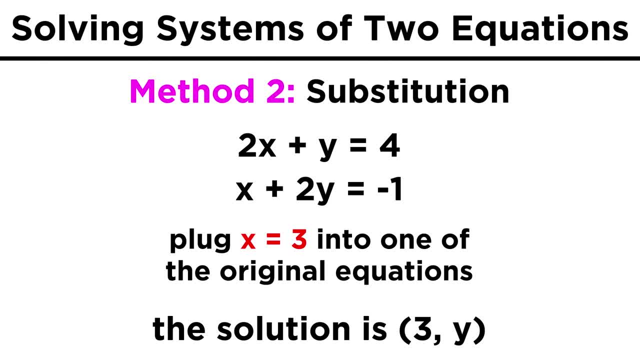 To get the Y value, we just plug this X value into either of these equations, Using the top one. two times three is six, and if six plus Y equals four, we can subtract six from both sides to get Y equals negative two. 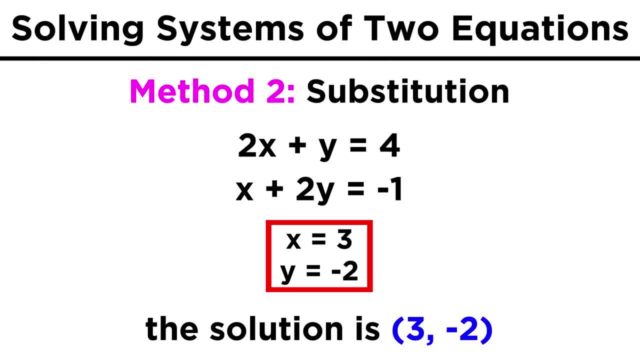 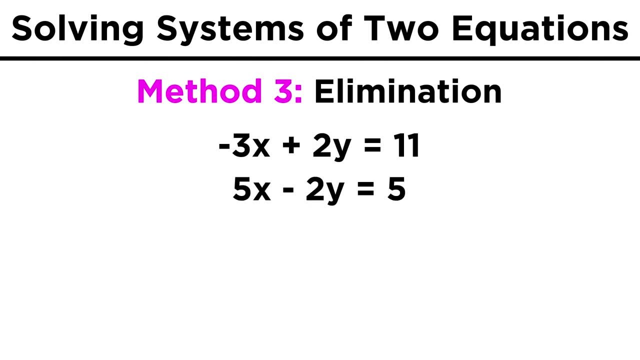 So X equals three and Y equals four. Two Y equals negative two or the point three negative two is the unique solution to this system. Substitution isn't the only technique we can use. We can use another technique called elimination. Say we have another set of linear equations. 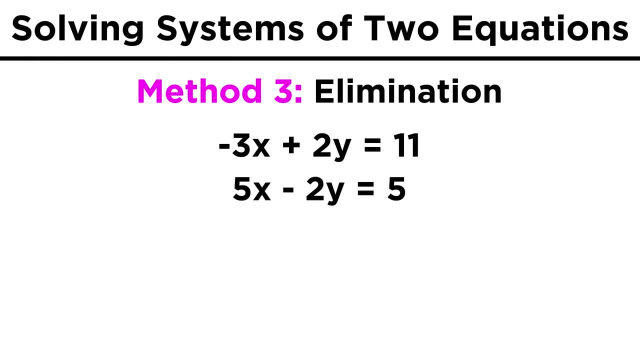 Negative: three X plus two Y equals eleven, and five X minus two Y equals five. Once again, we absolutely can use the substitution method. It's easier to go another route. We can combine these equations in such a way so as to get a new one where one of the variables 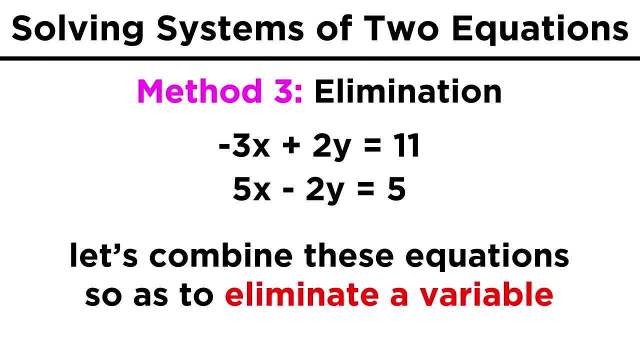 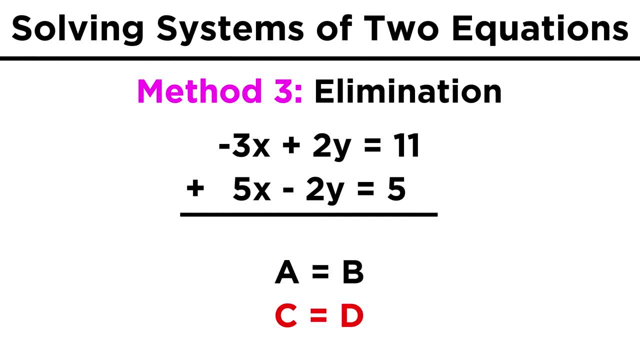 has disappeared. To do this in this particular case, we just add the equations together. This is valid because if A equals B and C equals D, then A plus C must equal B plus D. so we are just exploiting this logical truth to solve a problem. 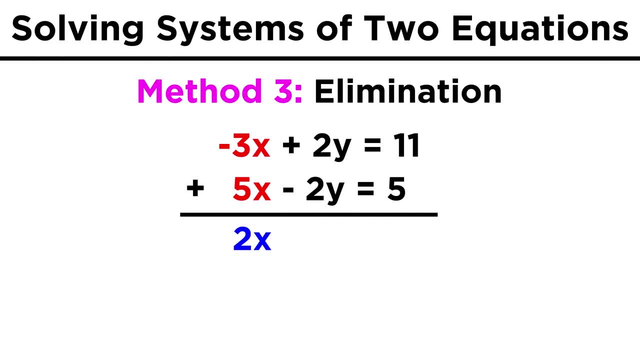 Negative three X plus two Y equals five. Negative three X plus five X gives us two X, Then two Y plus negative two Y gives us zero. The Y term goes away, and eleven plus five gives us sixteen. so dividing by two X equals. 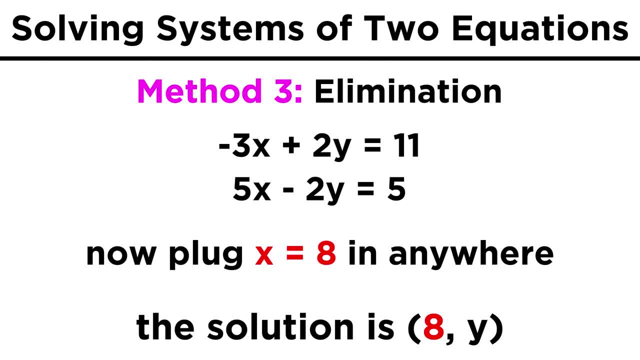 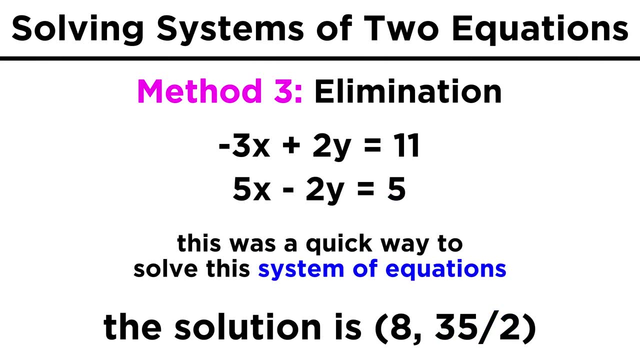 eight. Then we can plug eight into one of these, like the bottom one. We get forty minus two. Y equals five negative two, Y equals negative thirty-five and Y equals thirty-five halves. This was a pretty fast way to solve this system. 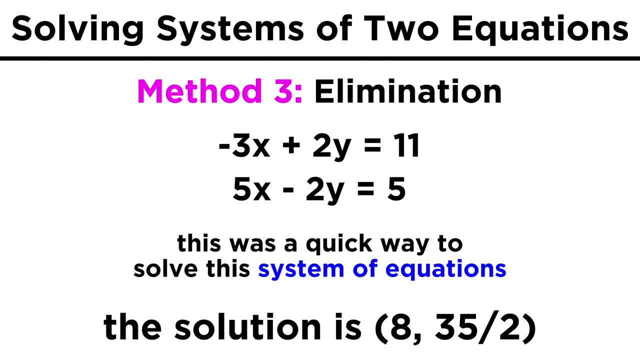 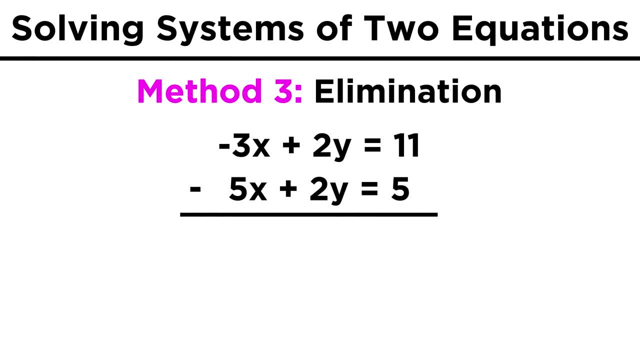 Of course it won't always be as easy as just adding them together. Sometimes we will have to subtract. If both of the Y terms were positive, we would subtract one from the other to get the Y terms to go away, and we would then have to be careful with our arithmetic, making sure we get the 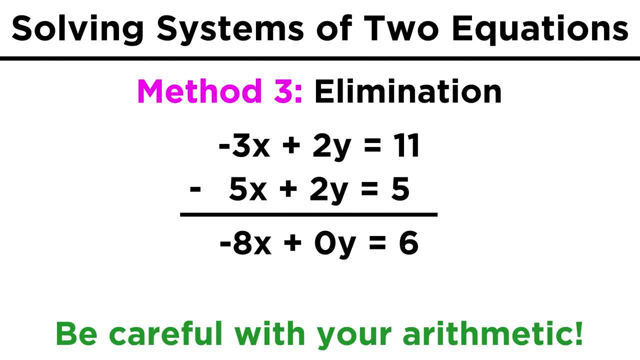 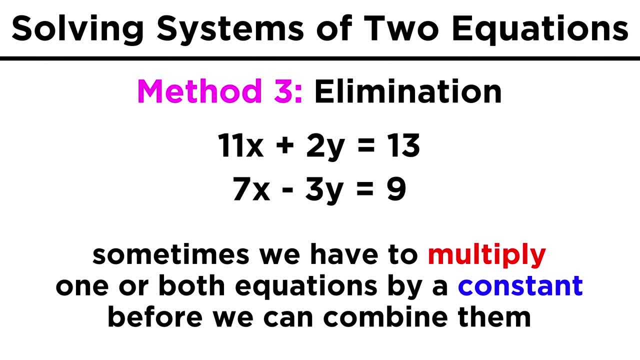 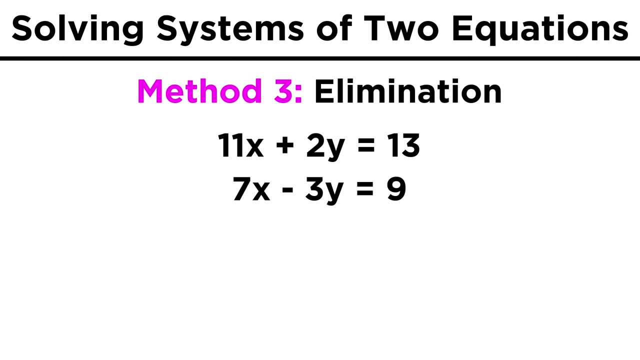 right sign on all the values in the answer. Furthermore, we might have to multiply. Multiply one or both of the equations by some constant to be able to do elimination. Say, we have eleven X plus two Y equals thirteen, and seven X minus three Y equals nine. 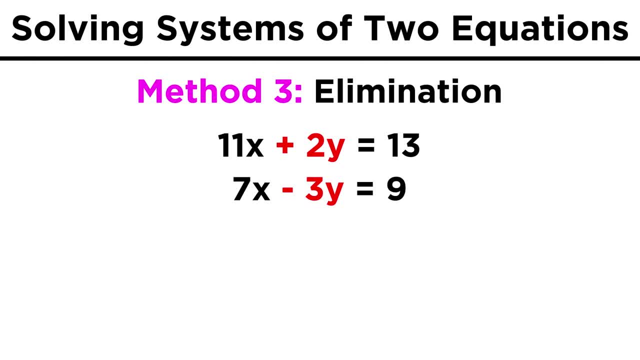 The Y values are pretty close, but we can't add them together as is and have them cancel. Instead, we have to realize that the least common multiple of two and three is six. So we multiply the top equation by three and the bottom equation by two. 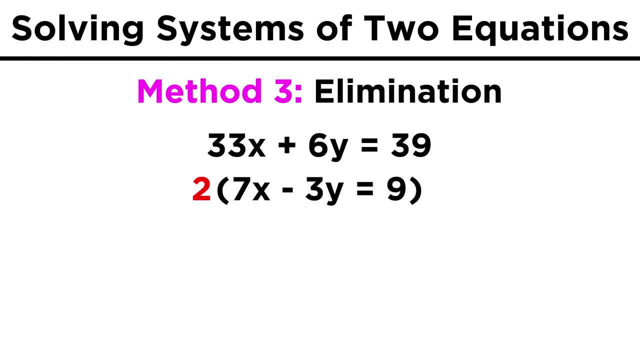 That gives us thirty-three X plus six Y equals thirty-nine, and fourteen X minus six Y equals eighteen. Now we are ready to combine them, because positive six Y and negative six Y will indeed cancel each other out. That gives us forty-seven X equals fifty-seven. 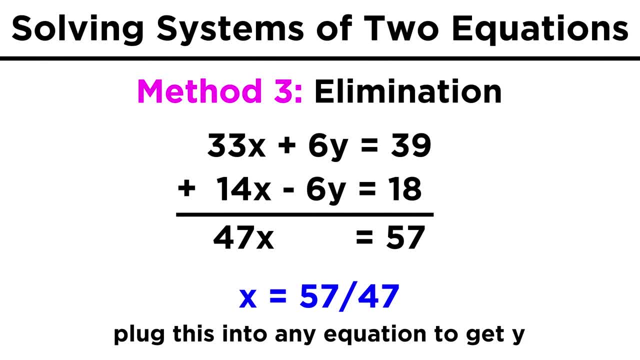 We can then solve for X and plug back into one of the equations to get the Y value. With lots of multiplying the solutions can get measured. We can then solve for X and plug back into one of the equations to get the Y value. 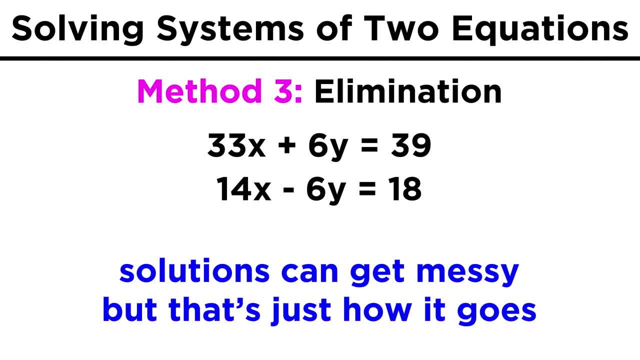 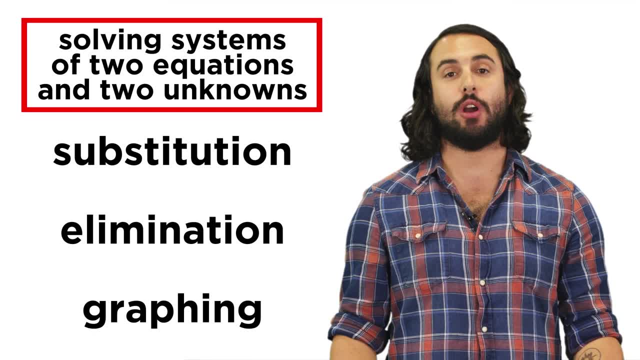 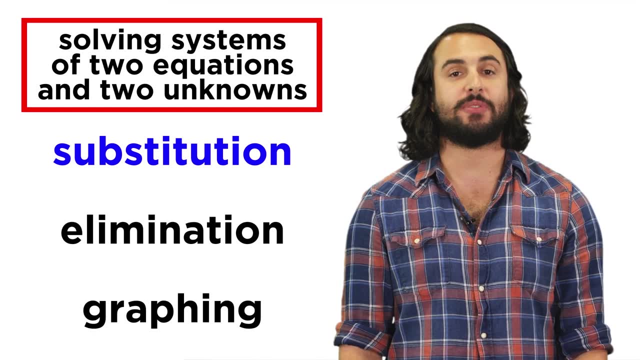 With lots of multiplying, the solutions can get measured, But that's just how they go sometimes. So, in summary, we can see that we have three options available to solve for a system with two equations and two unknowns. We can either use substitution by solving for one variable in terms of the other and 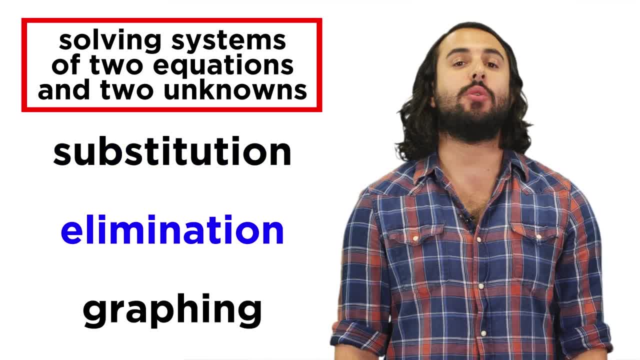 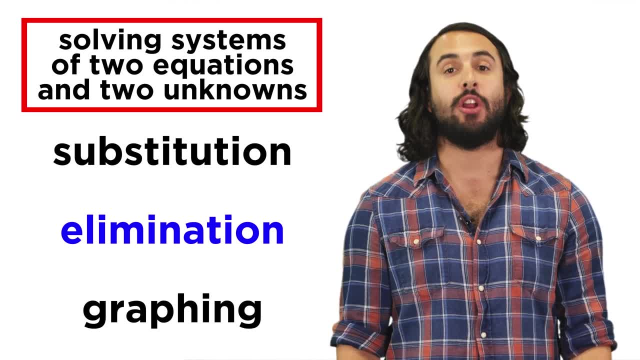 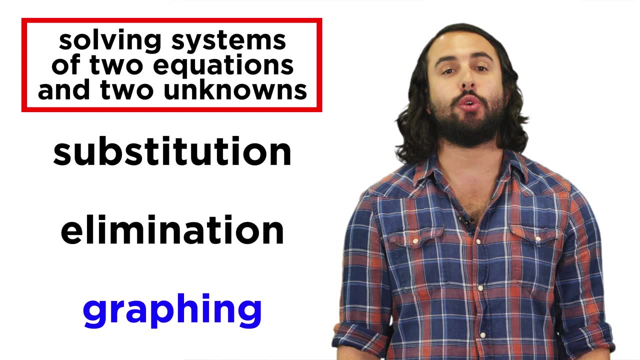 plugging that into the other equation. We can use elimination by manipulating one or both of the equations in order to combine them in some manner so as to get one, Or we can just graph everything and see where the two lines cross. If they cross once, there is one solution. 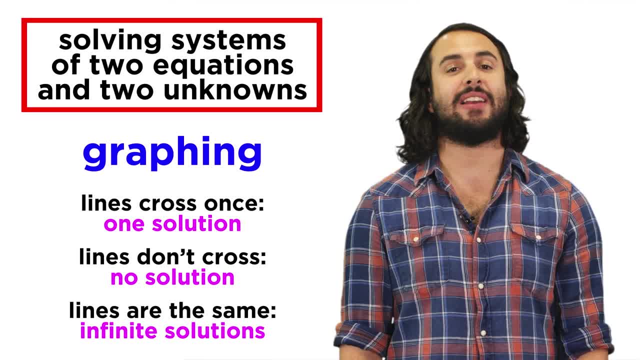 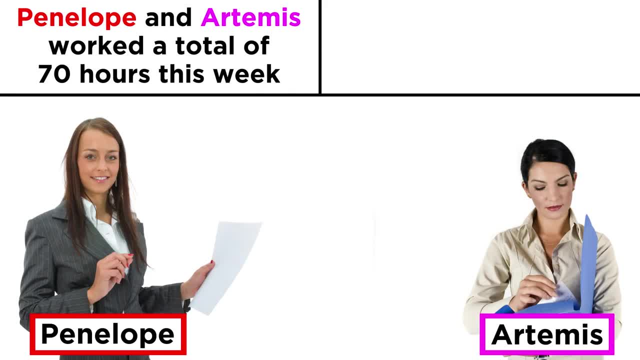 If they don't cross, there are no solutions. If they are the same line, there are infinitely many solutions. So why is this useful? Let's look at a real-world example. Say that Penelope and Artemis worked a total of seventy hours this week. however, Penelope 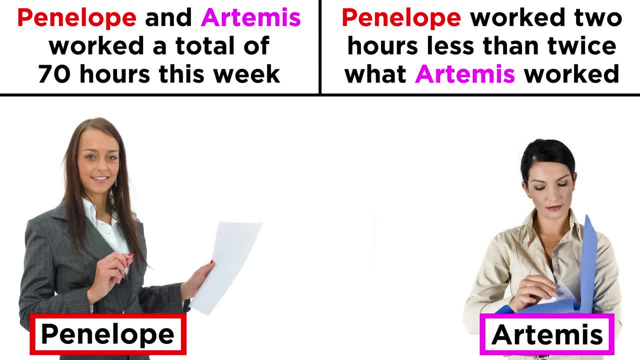 worked two hours less Then twice the number of hours that Artemis worked. How many hours did each of them work? While this example is relatively simple and if we did some guessing and checking we would eventually find the answer, that wouldn't be doing algebra. and if we learn the algebra? 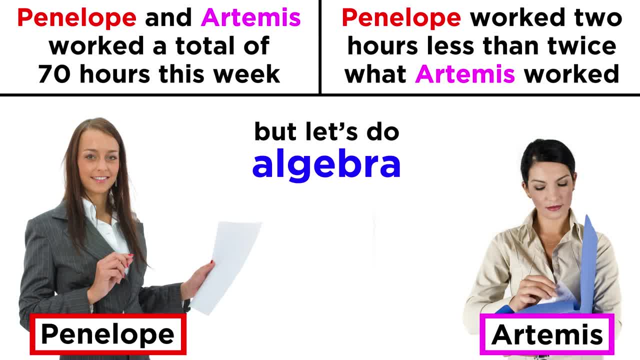 we can apply it to much more complicated systems where guess and check just isn't an option. First let's write some equations. The two of them worked a total of seventy hours. So let's write: P plus A equals seventy. Then we know that Penelope worked two hours, less than twice what Artemis did. 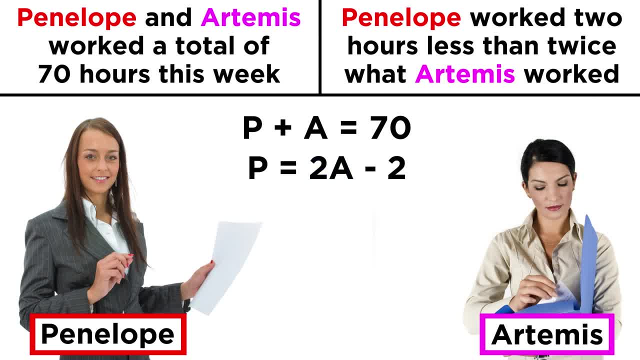 So P must be equal to two A minus two. There's our two equations with two unknowns. How shall we solve In this case? substitution seems pretty easy. as we've already solved for P in the bottom equation, Let's put two A minus two in the place of P in the top equation. 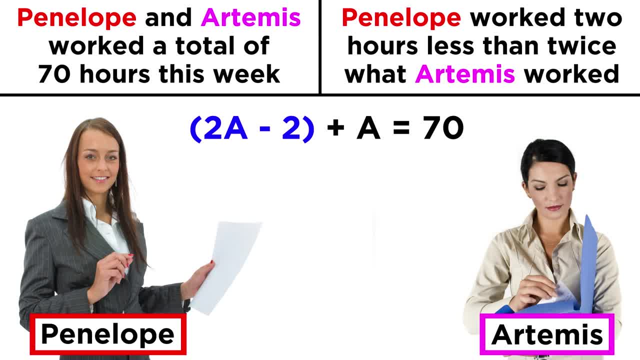 So let's write: P plus A equals seventy. That gives us two A minus two plus A, or three A minus two. on the left, We add two to both sides, divide by three and we get A equals twenty-four. Then we can use either of these equations to find P. Two times twenty-four is forty-eight. 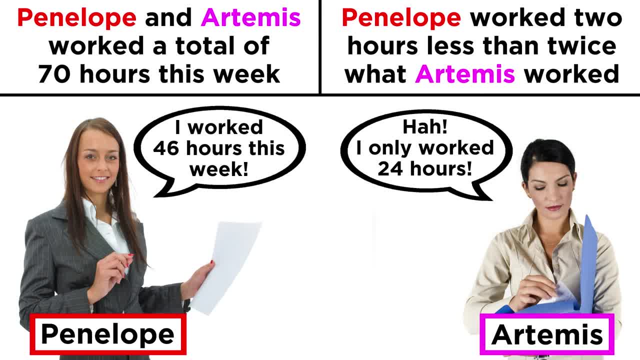 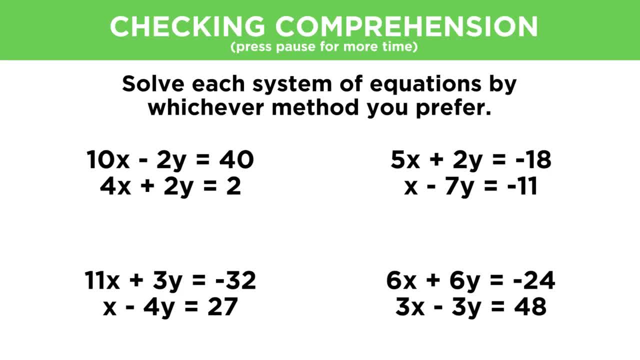 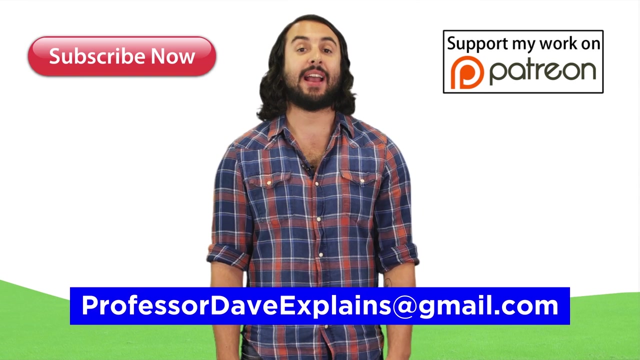 minus two is forty-six, So Penelope and Artemis worked twenty-four and forty-six hours this week. Let's check comprehension. Thanks for watching, guys. Subscribe to my channel for more Bye tutorials. support me on patreon so I can keep making content and, as always, feel. free to email me.